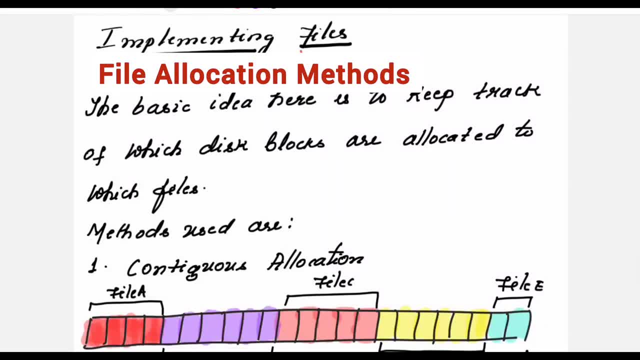 Hello viewers, welcome to this video lecture series on operating system. From this session onwards I shall discuss few topics on file system implementations. The very first topic here is implementing files. So this topic, implementing files, you can also study under one more heading called as file allocation methods. The question in the examination can 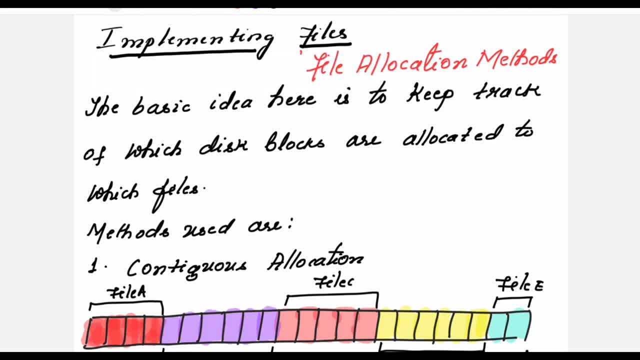 be like: explain the different file allocation methods. You are going to write the different file allocation techniques that are used here. So these techniques you are learning under the heading implementing files. So what exactly you mean by implementing files is see implementing file. the word implementing is used here because normally we can classify users into two types. 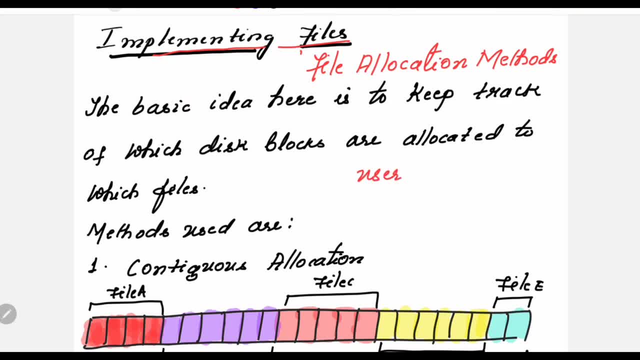 The first type of user who are just using or creating the file and all, and those users are only worried about what name to give to those file and what different operations that can be performed on the file. But for the people who are implementers, for them, the 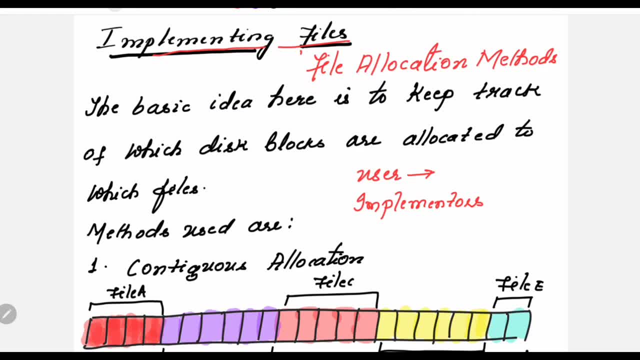 main thing is to give them the name of the file. So, for them, the main thing is to give the name of the file. So, for them, the main thing is to give them the name of the file. task is what, how these particular files get stored. i create a file called file one. the file one is: 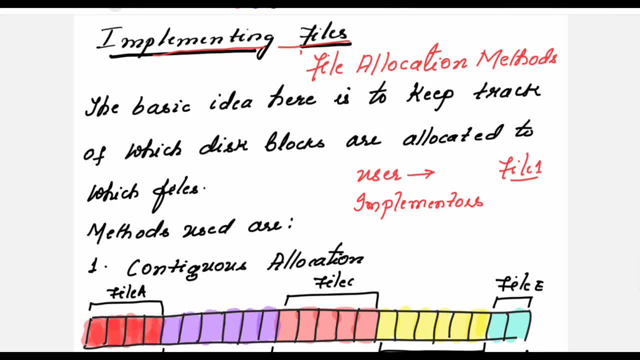 stored and saved into the disk. what is the method that is allocated here in order to store this file on the disk? so those things- that means those methods- comes under this heading, called as implementing files or file allocation methods. so this is what i said. just the basic idea is. 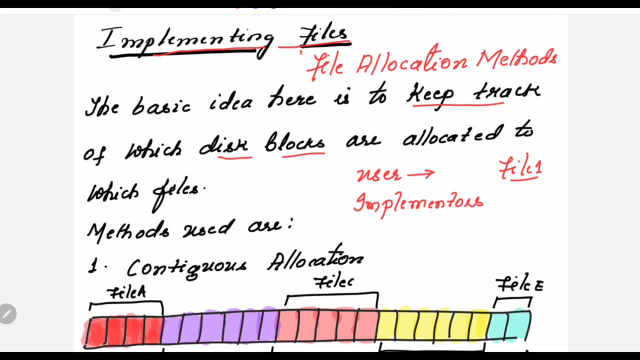 here to keep track of which disk blocks are allocated to which files, because your disk is having what? so many blocks, and in in that particular your disk is come. your disk consists of several blocks, so which blocks are used for which file? so if you are allocating this blocks, 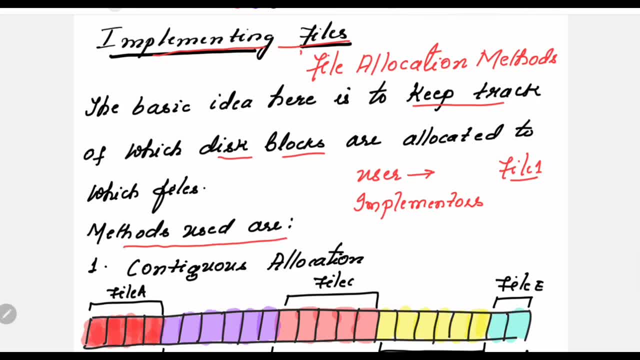 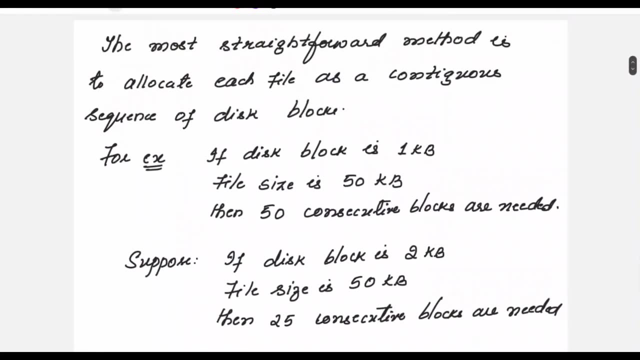 for one file. then what method are you using? because we have four different methods here that are used for allocation. the first one is called as the contiguous allocation. what exactly happens in the contiguous allocation, i shall explain. moreover, there is one illustration here. before that, let me tell you few things. 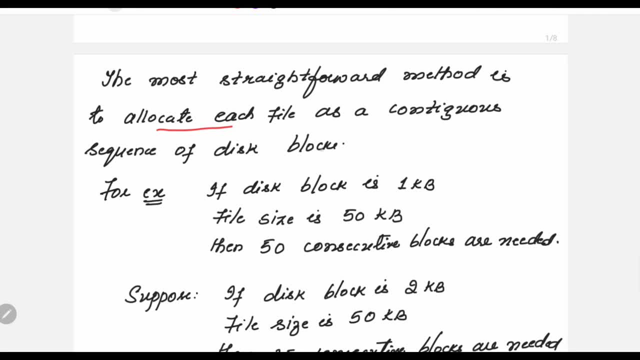 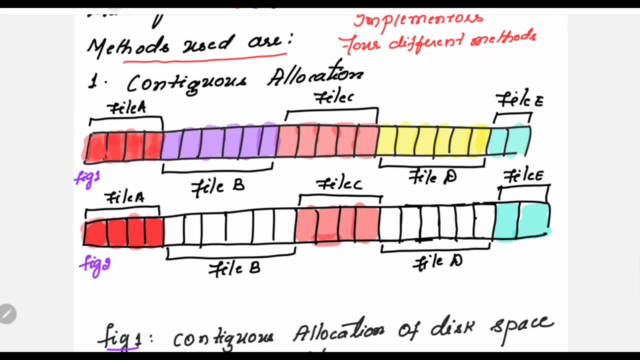 this method will allocate each file as a contiguous sequence of disk blocks. so this is what it is shown here in the figure. so initially the disk is empty. that means there are all these blocks are empty. here you start storing the file. file a gets created. the file gets stored. 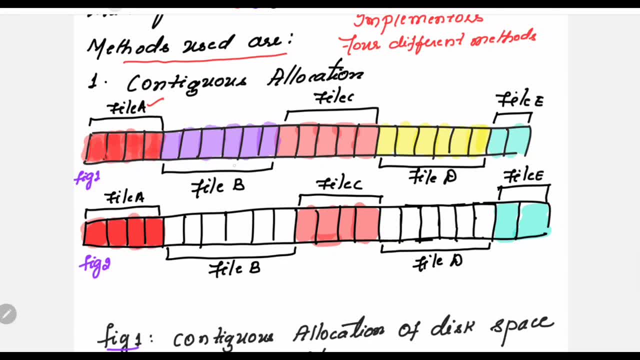 so it simply it is taking the first four blocks here. next, file b create gets created. it is taking how many? six blocks? and file c: one, two, three, four, five blocks. file d: one, two, three, four, five, six. so this way, one after the other, in a continuous manner, all the files gets stored. this method is 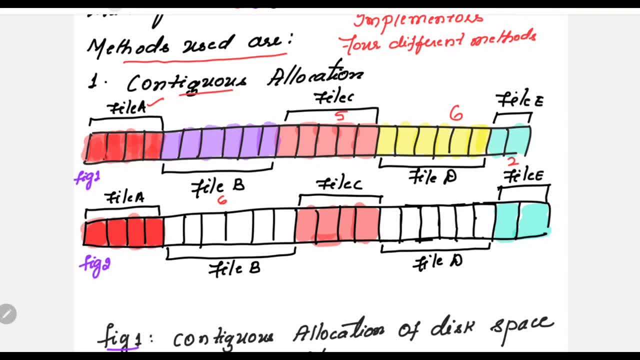 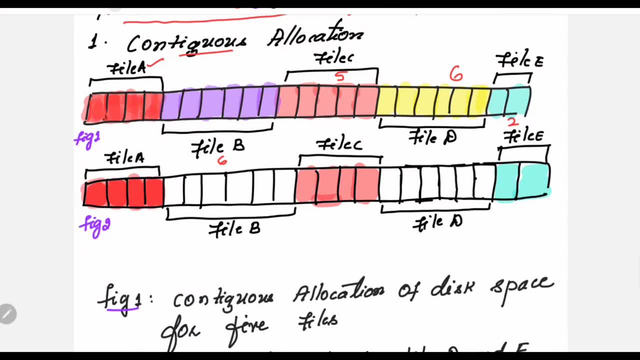 called as contiguous allocation. so in this method you should also see what type of advantage you can find here and is there any disadvantage? also, you need to check why we are allocating four blocks. it depends on the size of the file. see normally, if i am taking in simpler words, one block, one block. 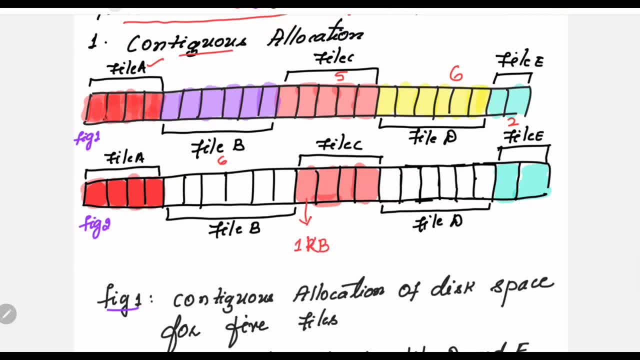 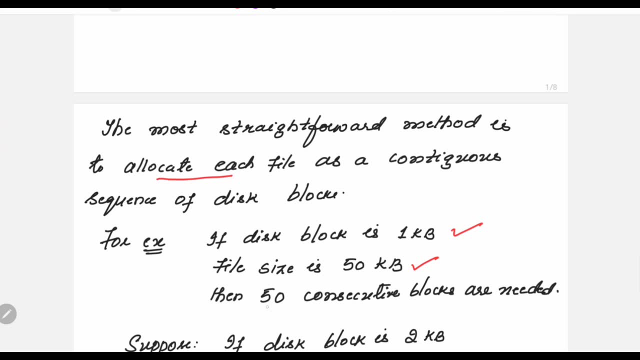 size. let me take it as one kb, fine, and if the file size is four kb, then what will happen? you need for four blocks here in in order to store this file c. so that is what i have written here. also, if the disk block is 1 kb, file size is 50 kb, then you need how many- 50 consecutive blocks are needed. 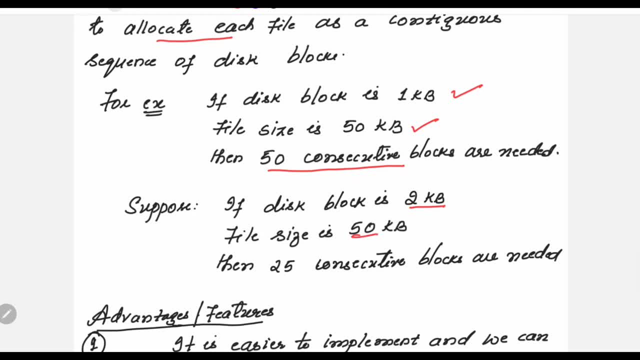 suppose, if you take the disk block size as 2 kb, file size as 50 kb, then 25 consecutive blocks are needed. so you are just storing in a consecutive manner all these files. in which type of allocation method? in contiguous allocation method. so what are its advantages? 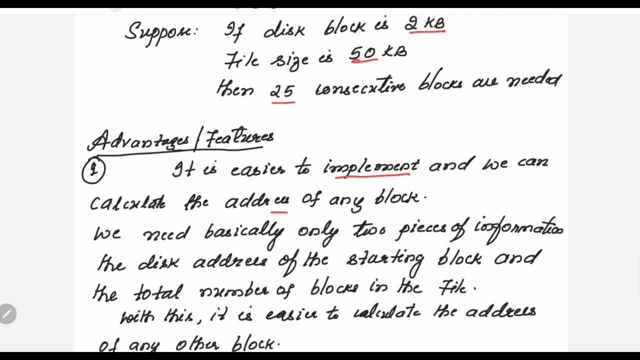 it is easier to implement the very first thing and we can calculate the address of any block. also, how do we calculate the address of any block? in order to calculate the address of any block, we need actually only two pieces of information. first thing is, we should know what is the. 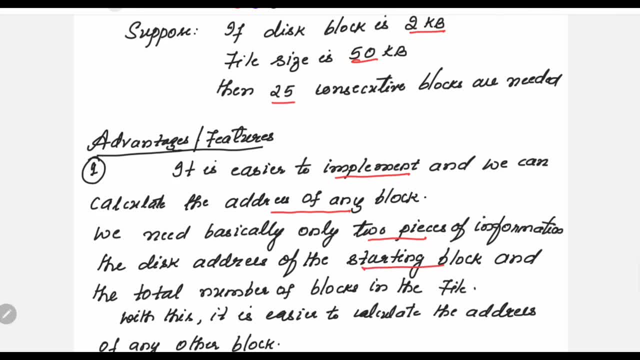 address of the starting block and how many blocks that particular file occupies. if you know these two pieces of information, then it is easier to calculate the address of any other block, for example. i'll show you here in this example. i'll show you here in this example. i'll show you here: 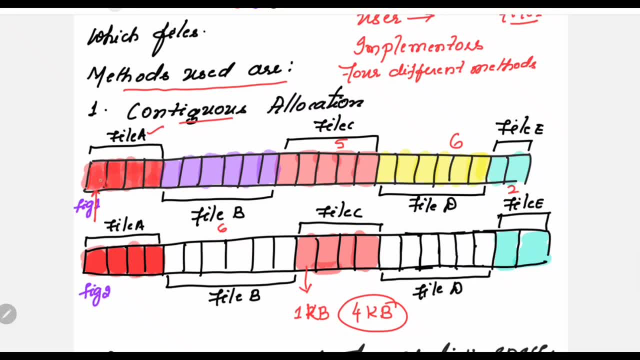 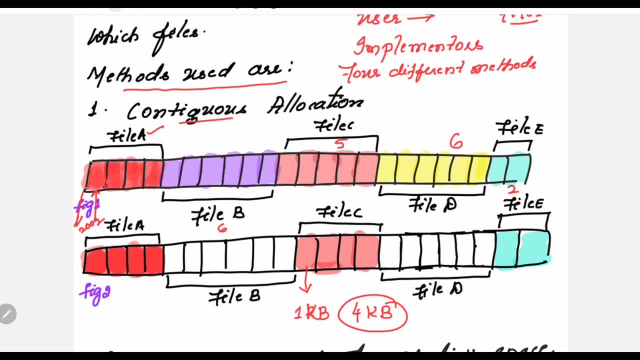 okay, we'll let us take. each block occupies two bytes of information, so the next one will take how much? the starting address is 2002, so it will end here. so it will start. the next block will start from 2004, the next will start from 2006, the next will start from 2008 and finally see the. 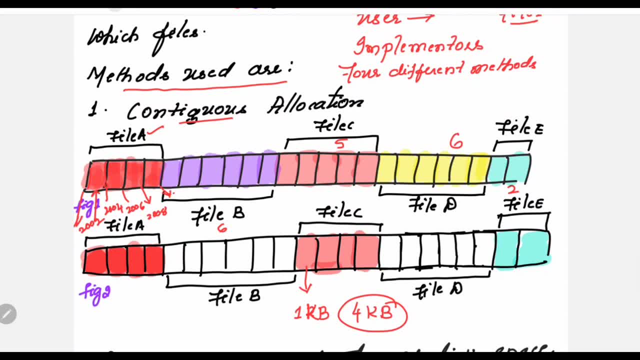 ending block is what it is: 2008. it will end at what: 2010. so 2010 becomes the starting address for the file b. so what ex? how did you arrive at the starting address of the next file is because you know the starting address of the first block and how many blocks this file occupies. let us take 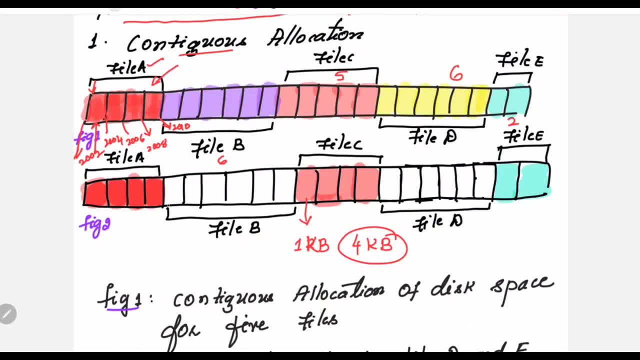 for example, the file gets removed from the disk. so here i am just showing one example. file b is taken away. fine, now you can see this is vacant, this is vacant, this is vacant. so these five blocks are vacant. next, file d gets removed. so you can see the next six blocks are vacant here. 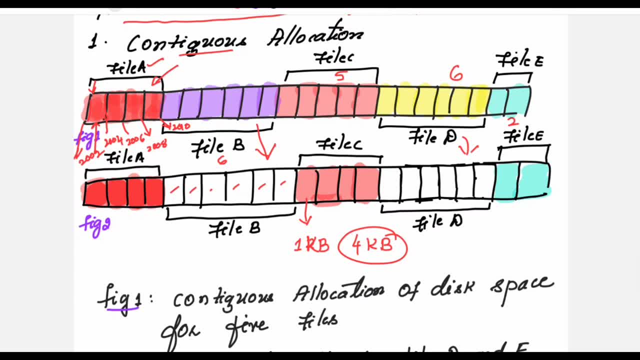 so this is one of the disadvantage in contiguous allocation method: as the file gets deleted, it leaves what the gaps in between. so these gaps, whatever gets created, will remain and we will always have what a disc is having, what a mix of files and gaps. files and gaps: one file, one. 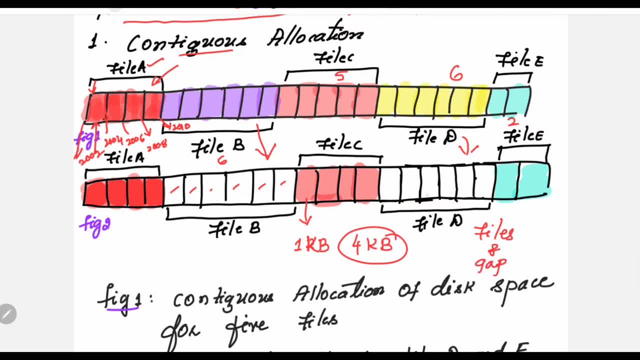 gap. so this is one main disadvantage in contiguous allocation method and we cannot even carry out the compaction here, because compaction is what: bringing all the gaps together at one place and bringing all the files. compaction needs more effort. it will take more time also because there 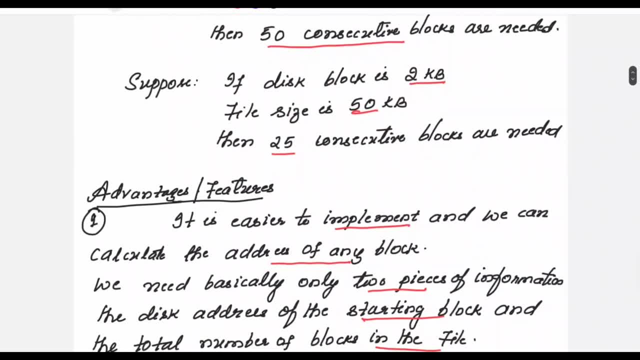 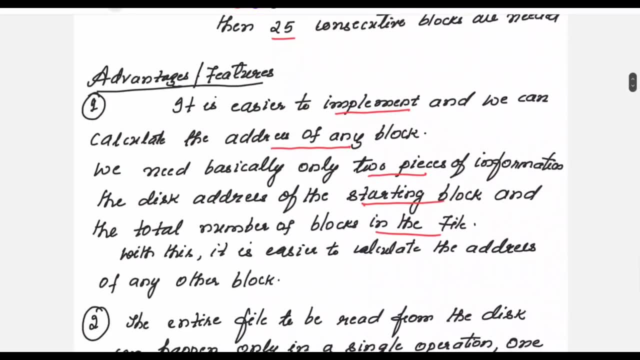 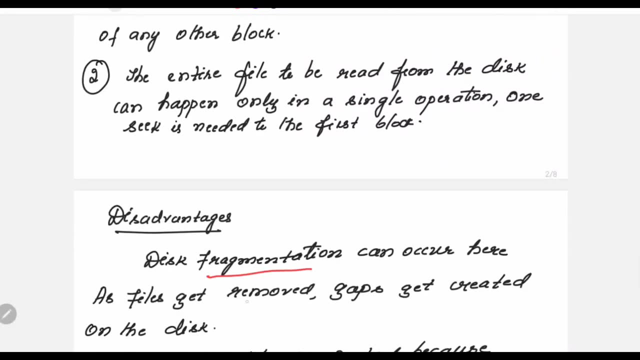 can be millions of blocks available on the disk. so this is one of the disadvantage. so we say normally when this kind of gaps gets created in the disk there is a fragmentation happening. So I have written here the disadvantage. The disk fragmentation can occur. as files get removed, gaps gets created on the disk. The disk cannot be compacted. also, 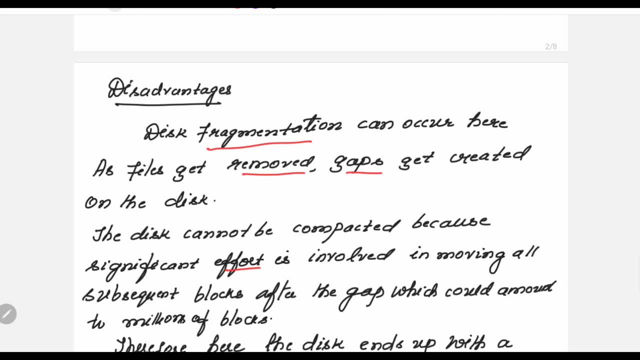 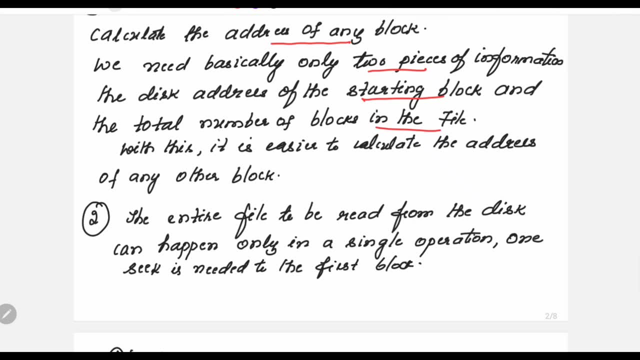 because significant effort is involved in moving all subsequent blocks after the gap, which could amount to millions of blocks. The another advantage in this method is the entire file to be read from the disk can happen only in one single operation because only one seek is needed to the first block. So this seek time, hope you people are familiar. it is the time taken. 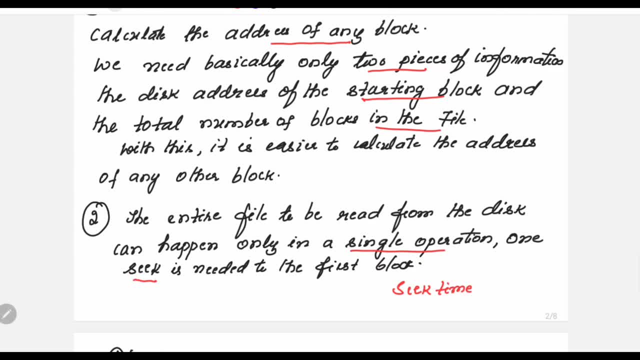 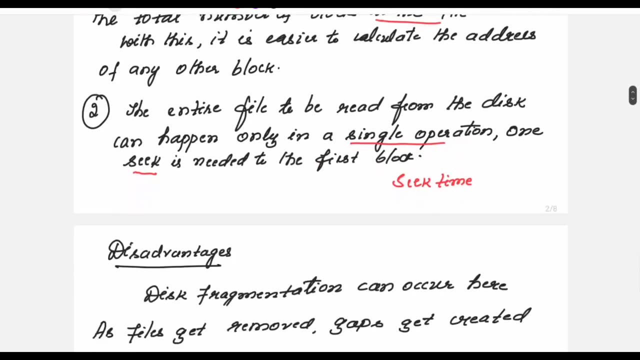 by the read write head to move from one track to another track, since all these are present in a continuous manner. So only one seek is needed, and that too to the first block Later on. automatically it will keep on reading the subsequent blocks. So this is the second. 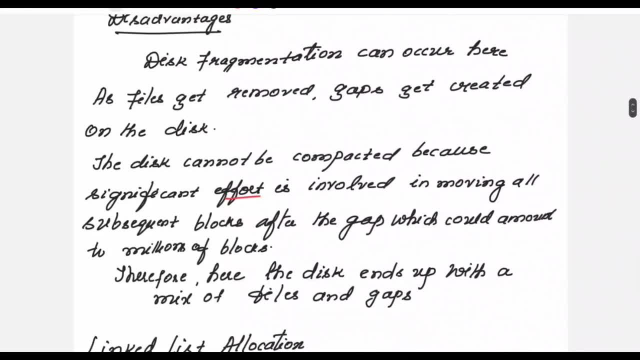 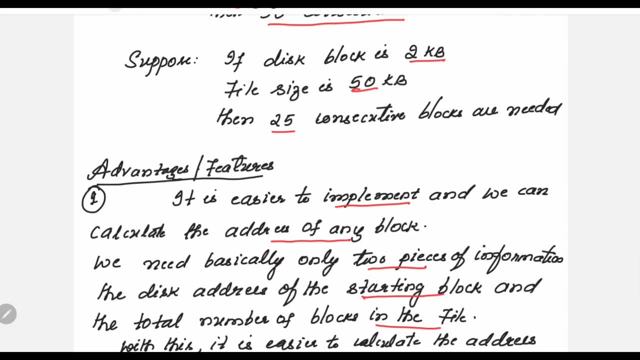 advantage and disadvantage. as I already told you, the disk fragmentation will occur here. That is, even though in the question, if the word advantages is not asked in the features, that is, in the description or in the working of that method, you can write this advantages also, Then only the. 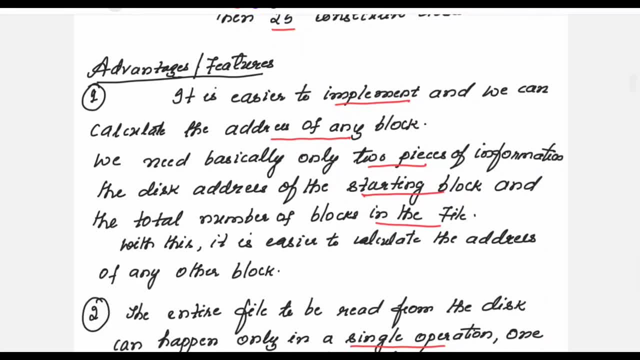 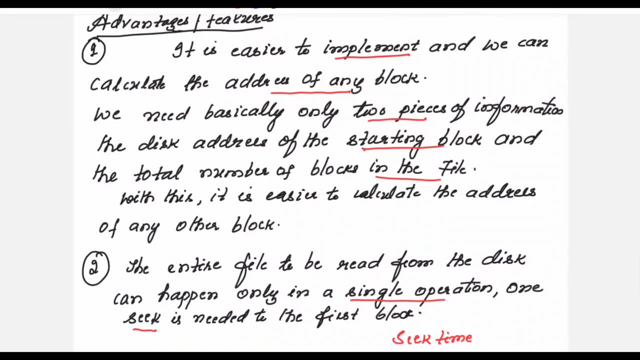 explanation gets completed Specifically. if advantages and disadvantages are mentioned, then also you are going to write these things. So mainly two advantages are there. The first one, as I said, it is easier to implement also and easier to calculate the address of any other block. 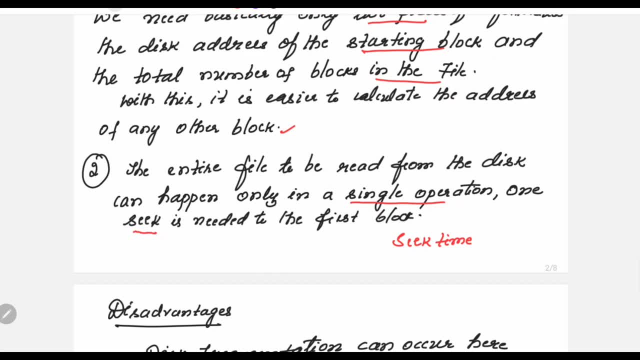 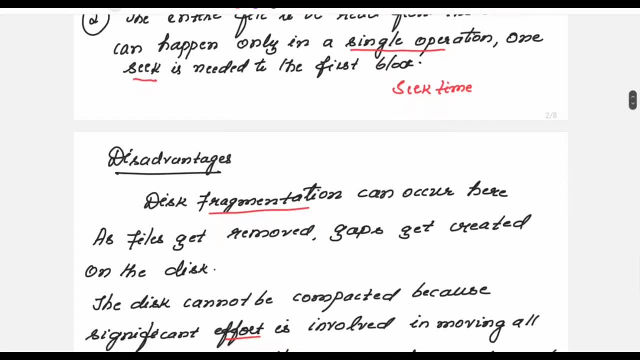 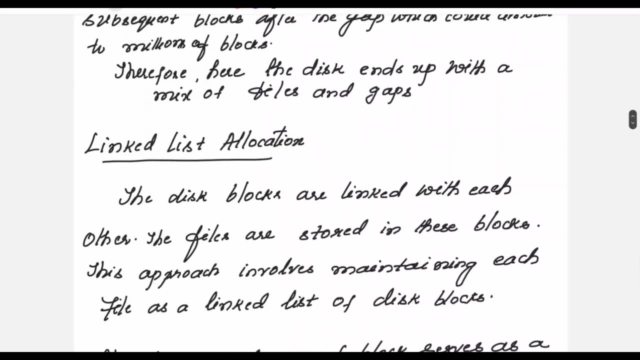 And the second and main advantage is it needs only one seek. That means by just one single operation you can read the entire file, and in disadvantages, this fragmentation will occur. So now let me move to the next method, that is, the link list. 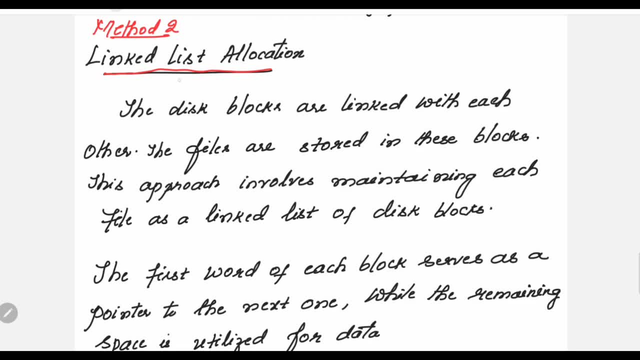 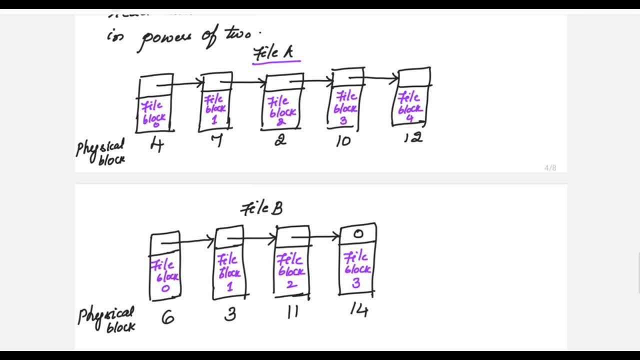 allocation method. So this is the method two. The name of the method is link list allocation method. So let me show you this link list allocation method with an illustration. What exactly is shown here in the diagram is there are two files, file A and file B. okay, If you. 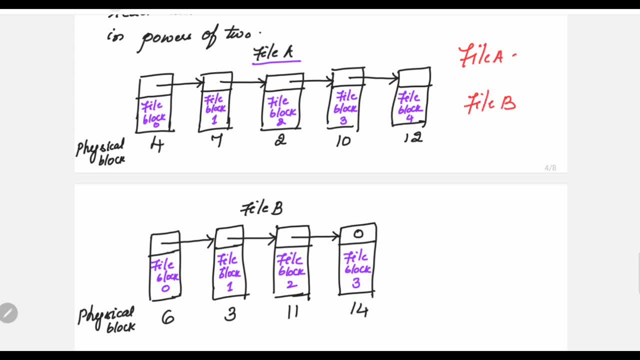 see here file A occupies how many One, two, three, four, five blocks and file B needs one, two, three, four blocks. Now, in the previous allocation method, that is, in the contiguous allocation method, we have seen that whenever a file is removed it leaves the space. That means 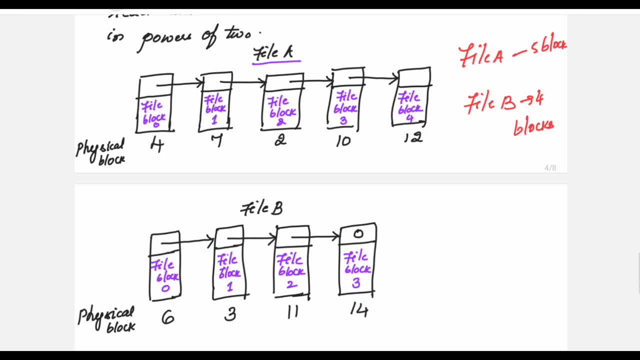 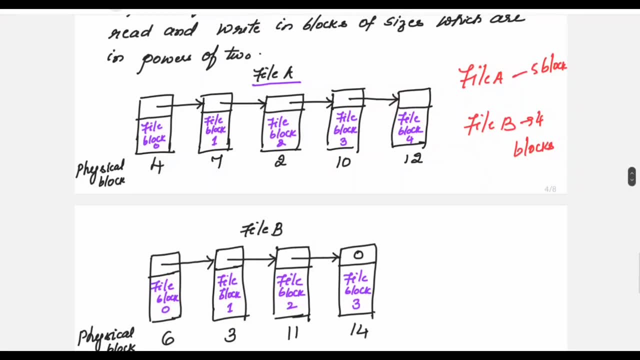 disk fragmentation was occurring. And even when we try to create a new file, then the new file size may not match with the existing fragmentation that has occurred. For that reason we are going for the second method. We call this second method as link list allocation method. So wherever are the free blocks available? free disk blocks. 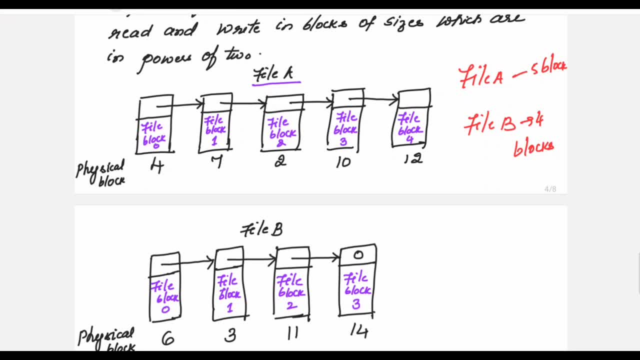 available. those blocks can be used, But how exactly it works? This is your block. okay, This is the block. So, in whatever manner you have stored earlier, same way: the contents of the file gets stored in this block, But some part of the block is used here to store. 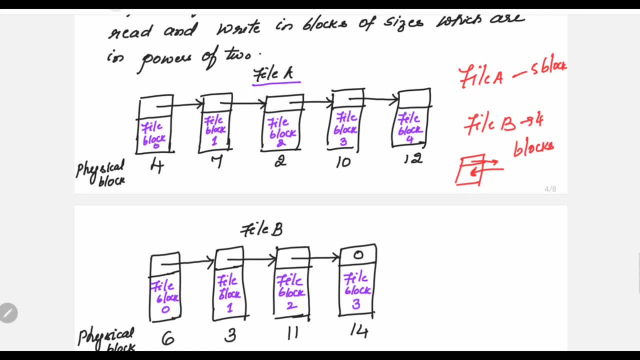 the address of the block which is next in the order. For example, you can see: these are the physical block numbers 1, 2, 3, 4,, 5, 6, 7,, 8,, 9,, 10, 11.. 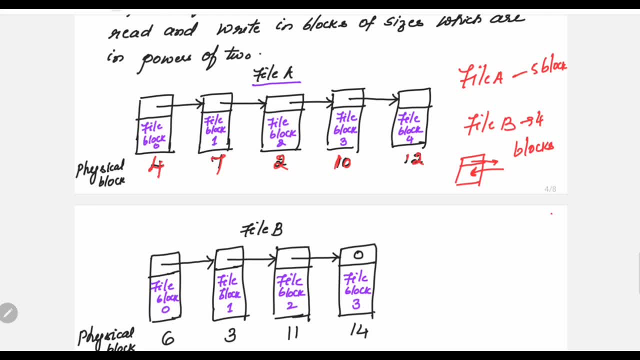 4,, 7,, 2,, 10 and 12.. Here block 4 is there. So the starting part of the file, that is, file block 0, gets stored in the physical block 4.. This file block 0 is also what it is storing. 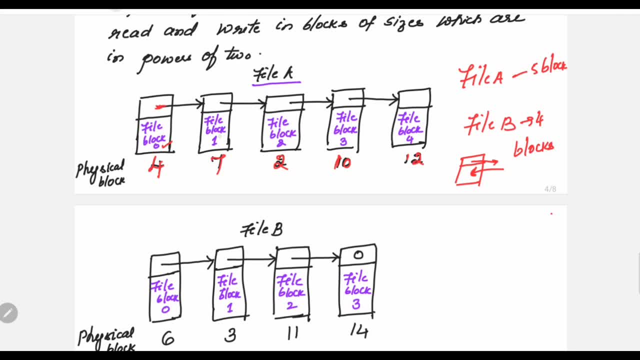 the address of the next block where the second part of the file is stored. We say that it has file block 1.. So file block 1 will point to the next block, wherein it will find the contents here present in file block 2.. So this way each block will 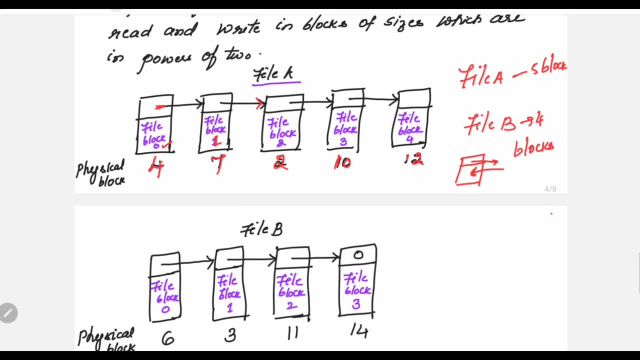 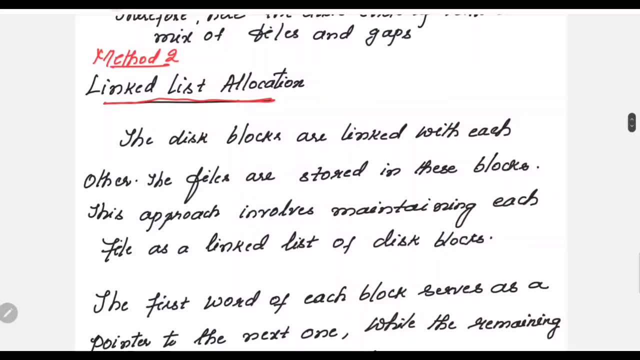 point to the address of the next block and you are able to use the disk space efficiently here. This is one main advantage. This is what I have written also here in the explanation. If you want, you can refer this video for notes as well. 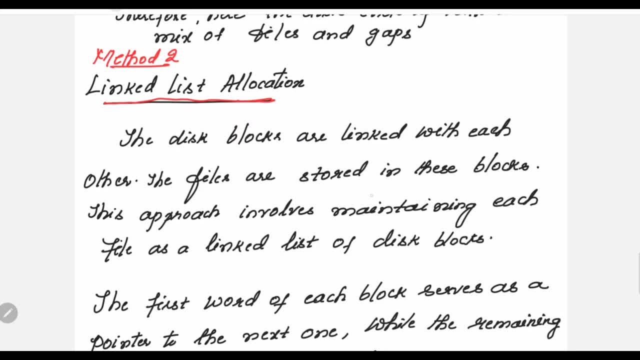 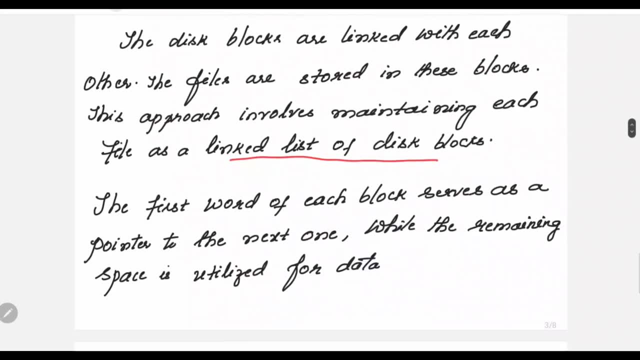 In linked list allocation method, the disk blocks are linked with each other. The files are stored in these blocks. This approach involves maintaining each file as a linked list of disk blocks. The first word of each block serves as a pointer to the next one, while the remaining space 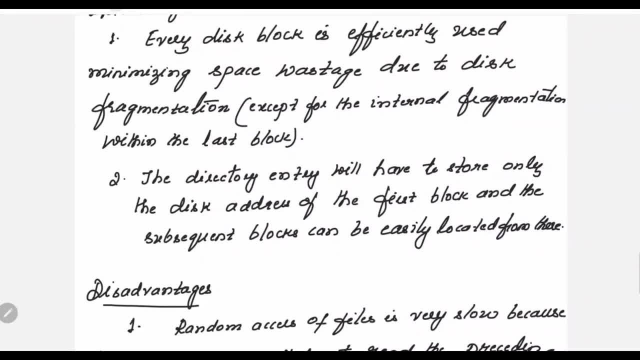 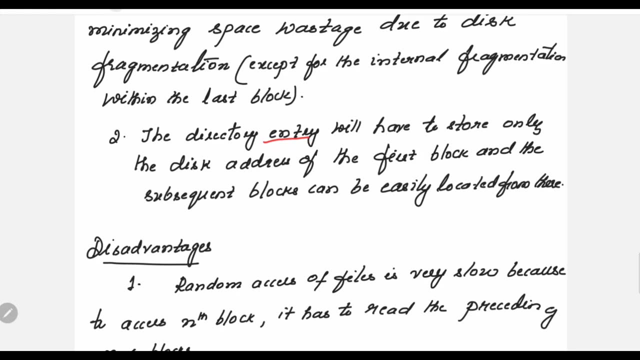 is utilized for the data. So, as I said, the advantage for this it is efficiently making use of the space, no wastage at all. but there can be an internal fragmentation within the last block that is quite oblivious. The next advantage is the directory entry will have to store only the disk address of 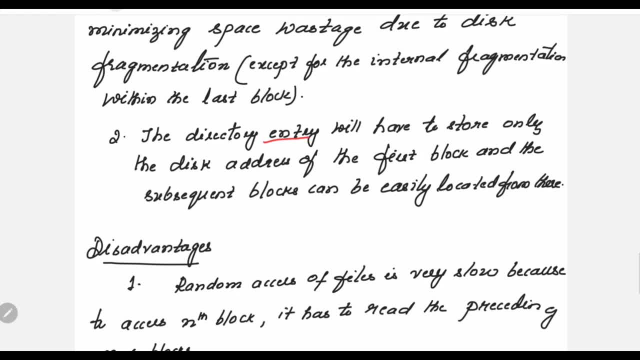 the first block and the subsequent blocks can easily be located. So one: you should also know that every time whenever a file is created, it is stored under one directory. So this directory will also have. This directory will store the information about the file. That means, if that particular file is there, file A, if this file A is having some 5 blocks. 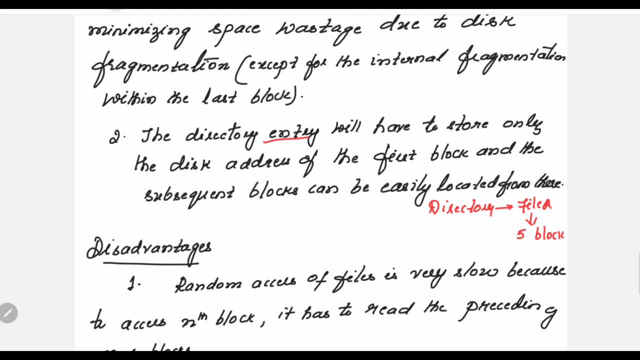 then the disk address of each of these blocks will be stored, Normally in the contiguous allocation method, but in linked list allocation method. no need to store the disk address of all the 5 blocks, just to store the address of the first block, because the first block itself will take you to the next. next. 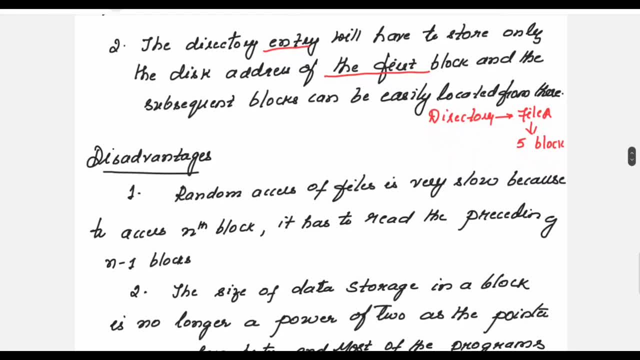 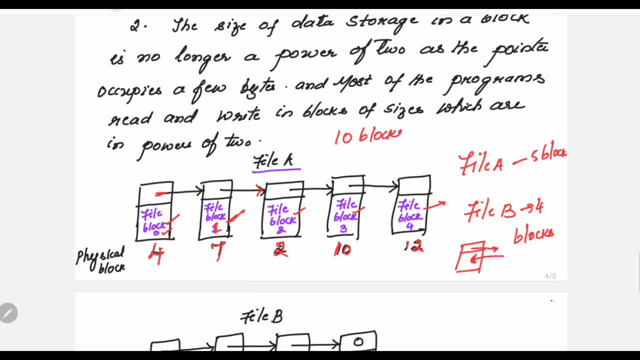 So subsequent blocks can be located from there onwards. This is the main advantage. The disadvantage of this is what if there are 10 blocks occupied by a file, then in order to read the 10th block, the previous 9 blocks must be read, 10 minus 1.. 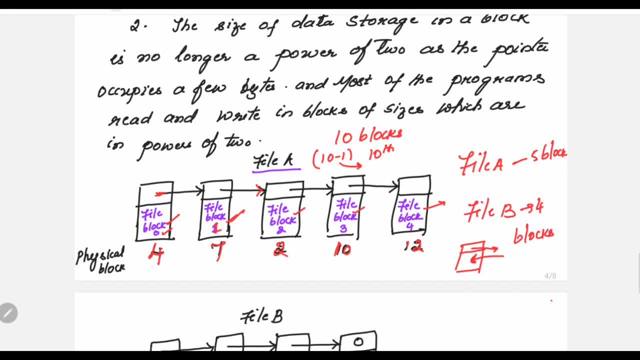 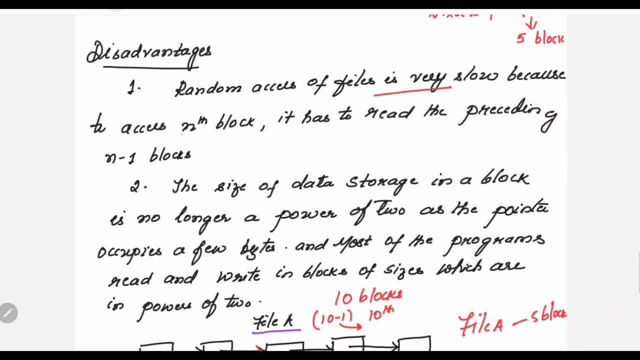 That means all the 9 blocks must be read first in order to reach to the 10th block. This is the disadvantage in this method. So we say the random access is very slow because in order to access the nth block it has to read all the preceding n minus 1 blocks. 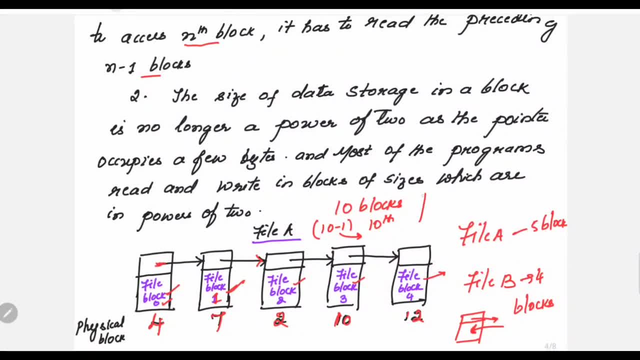 This is one disadvantage, and also the disadvantage is normally, when we have a block like this to store the data, always the data is stored in terms of what- the size of powers of 2.. But since now some part of the block is storing the pointer, that is, it is storing the address. 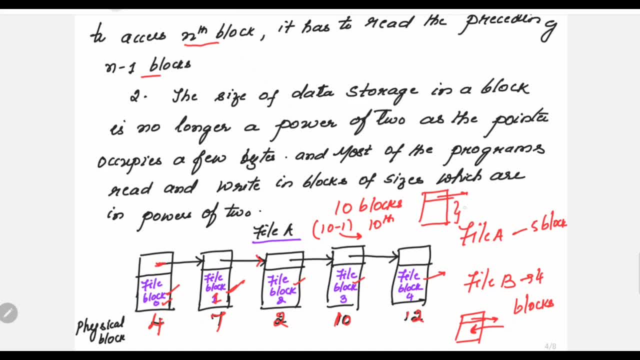 of the next block, the data cannot have a size in terms of powers of 2.. This is one disadvantage, because most of the programs will read and write in blocks of sizes which are only in terms of powers of 2. So this is the disadvantage. 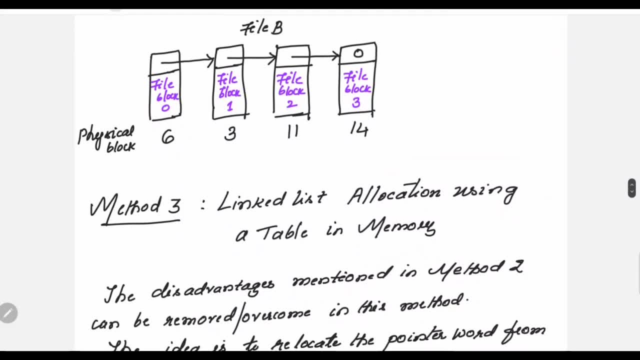 So this is the disadvantage. So that is about the second method. Now let us go to the third method: link list allocation method using a table in the memory. So earlier is link list allocation method, but this time it is what? link list allocation using a table in memory. 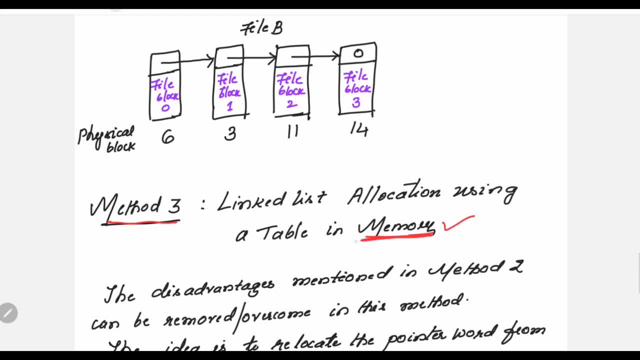 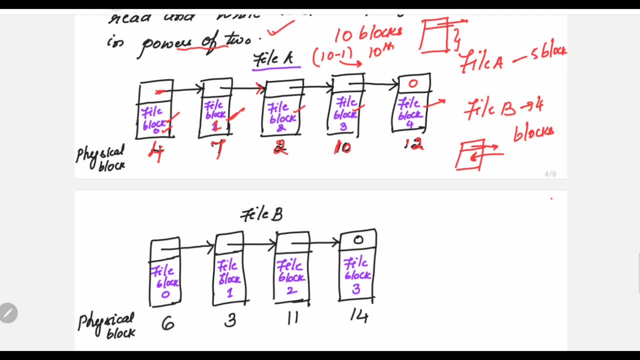 This is more important here: the word memory. Now, what you are going to do is you are storing whatever addresses. see this part, if you see, and moreover, yes, this 0 in the last block indicates it is the end of the file. Similarly here Here: 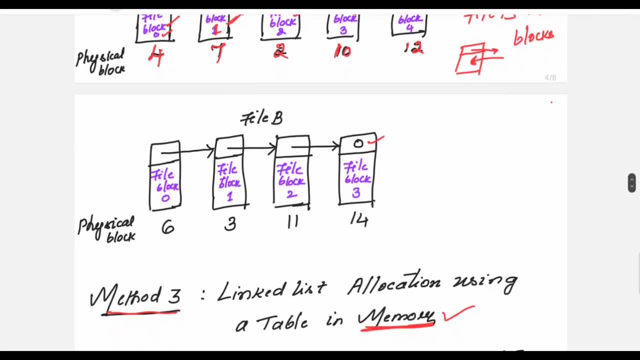 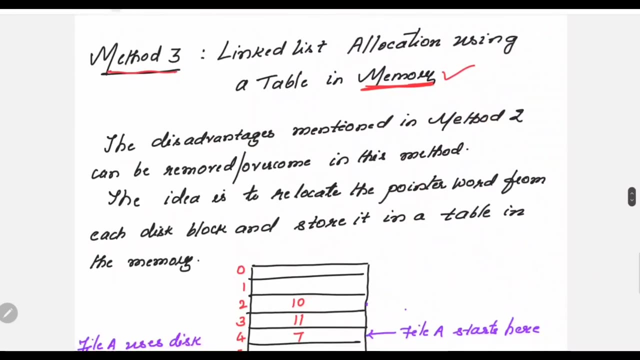 So here, in the previous method, that is, the link list allocation method, whatever space you are using here in order to store the address- okay, this now- no need to store the address in the block. instead, maintain a table wherein you are storing the addresses of all these blocks. 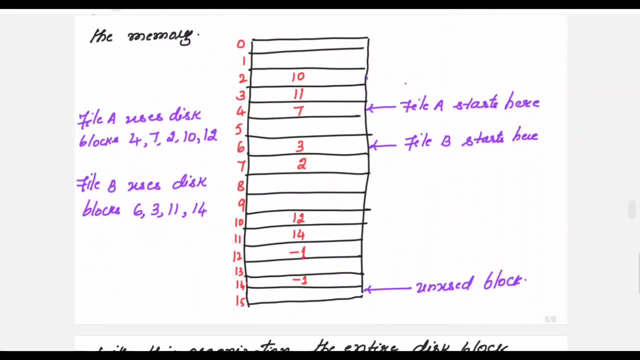 So this is what is here. the table is in this manner You can see. see we had there two files. file a was there. file a was using the physical blocks 4, 7, 2, 10 and 12.. So the address of all these five blocks will be stored here in the table. 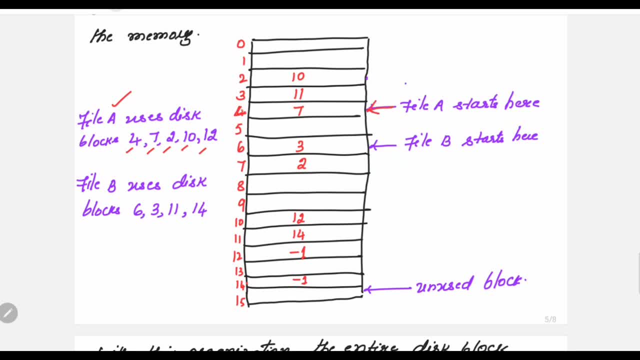 So this is what the file a will start from here, because the very first block is what block? number 4? when you reach this block 4, the content is what block 7? that means it is taking you to block 7.. Block 7, if you read the content, is 2, 2 will finally what 2 block 7 will take you to. then 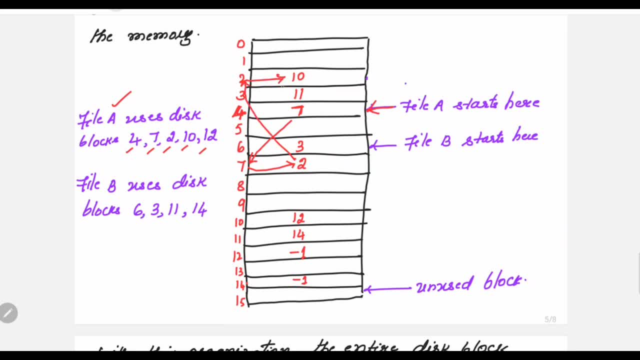 from 2 you are going to This block, then 2 will take you to the block number 10 and the block number 10 will take you to block number 12.. So this way you are able to access randomly any block of that particular file. 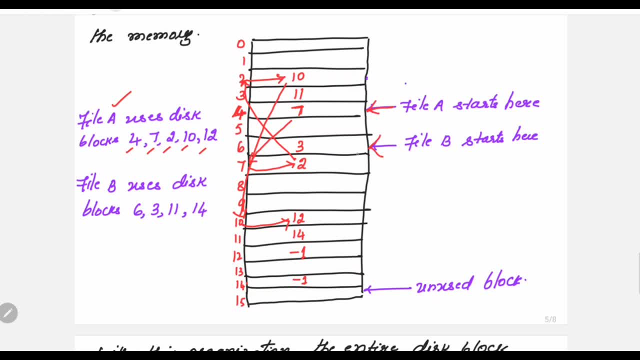 So here in this example we have shown file b also. file b starts from here, you can see. file b is using this block: 6, 3,, 11 and 14. file b starts from here, you can see- is using the block number 6,, 3,, 11 and 14.. 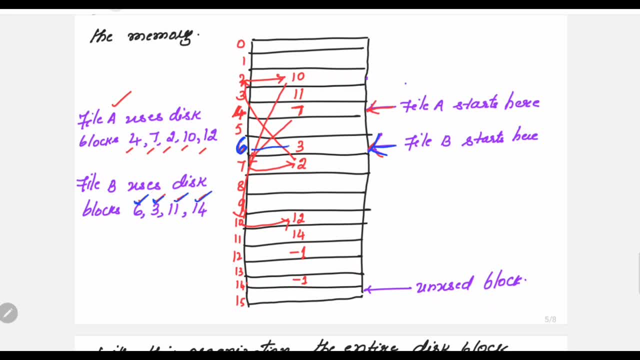 So here you can see the block number 6,, 3,, 11 and 14.. So first it will go to 6,. 6 will definitely say that you have to go to block 3.. So it will go to block 3. then block 3 will say that you need to go to 11.. 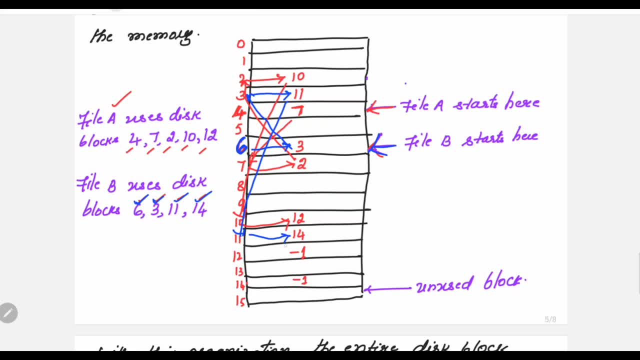 So 11 will say that you need to go to 14 and from 14, when you go back, definitely you will see what minus 1, minus 1 indicates. what is the end of the file? So here, previously for file a, this is the end of the file, while for file b, this is the. 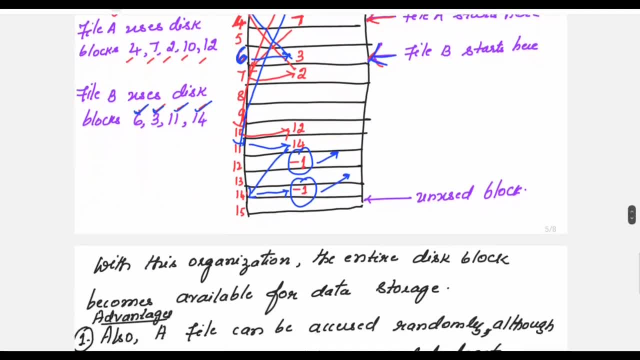 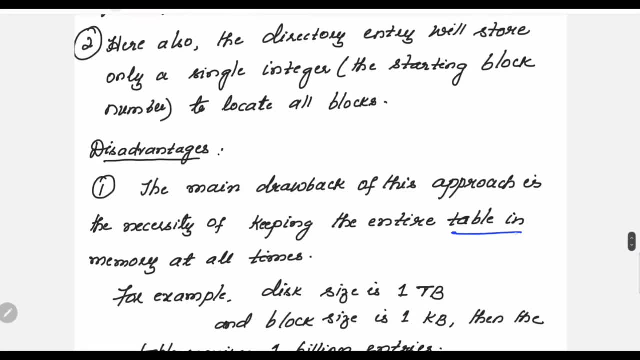 end of the file. So definitely we see an advantage. So this is the end of the file. So definitely we see an advantage here because we are able to randomly access any block. but what about the disadvantage? The main disadvantage is to keep the entire table in the memory at all times. 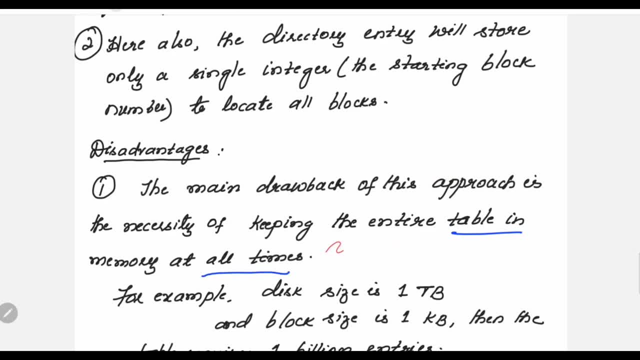 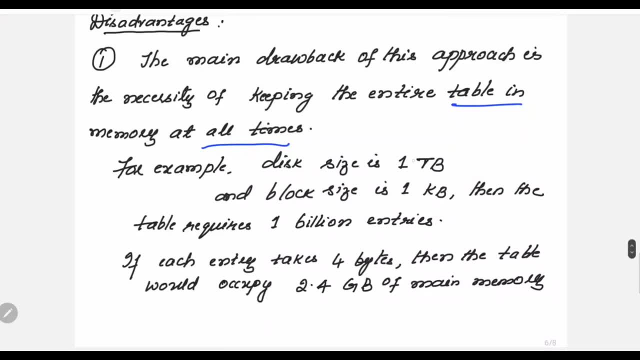 Main memory is very precious. if you are keeping the table in the memory, then what about the space that it takes in the main memory? One example I have shown here. let us take the disk size as 1TB. block size is 1KB, then you need to store the addresses for each of these blocks. 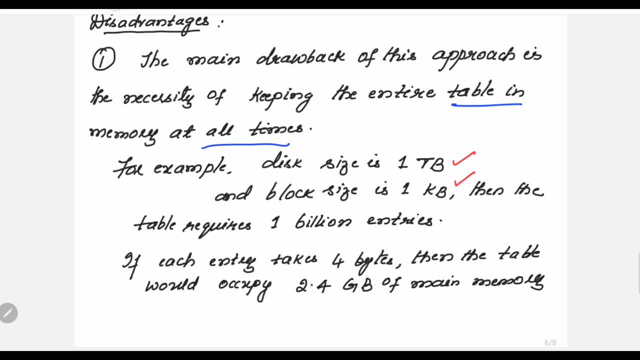 So then, when you are storing the addresses for each of these blocks in the table, the table will have 1 billion entries. and also you should not forget that each entry may take some bytes, like 3 bytes or 4 bytes. So suppose if it is taking 4 bytes to store the entry, then the table will take how much. 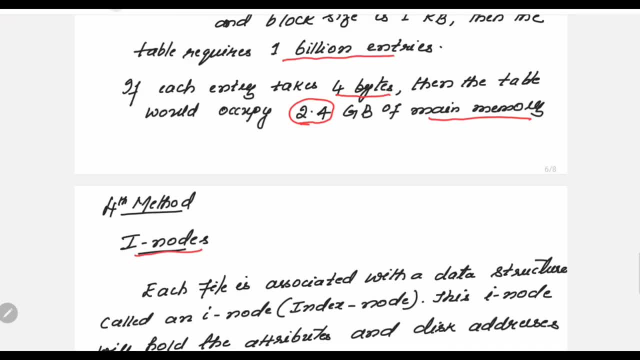 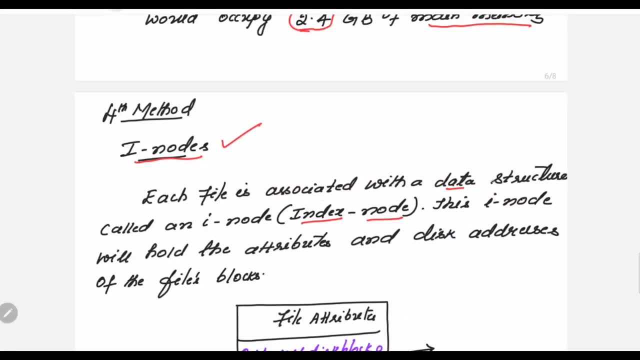 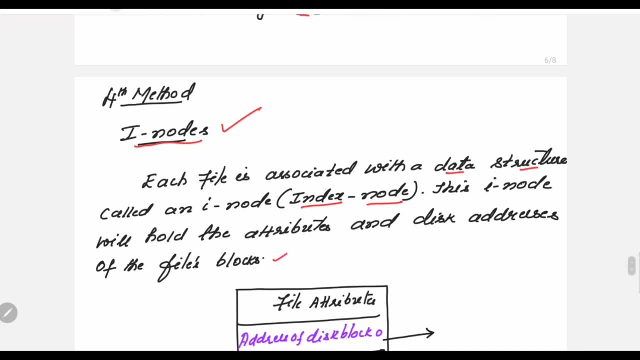 2.4 GB of the main memory. The fourth method is the inode method. inode- i stands here for index node. in this method each file is associated with it. Each file is associated with a data structure called inode. So this inode will hold the attributes and disk addresses of the files. block. 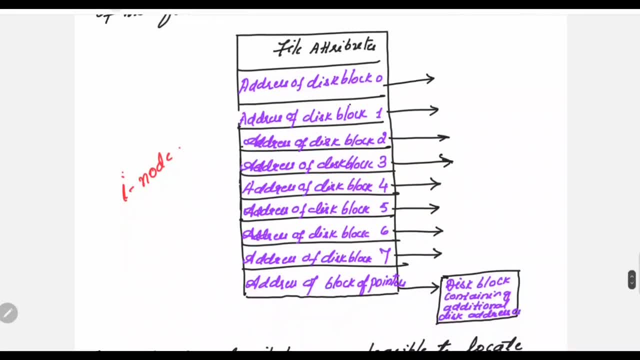 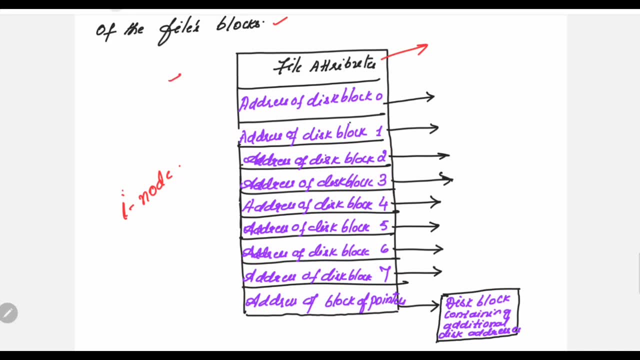 So every file is associated with an inode. and what does this inode consist of? one example I have shown here. you can see for that file. first suppose let us take for example, this is some file p or file p. File p is having some 8 blocks, then the addresses of each of these blocks are stored in this. 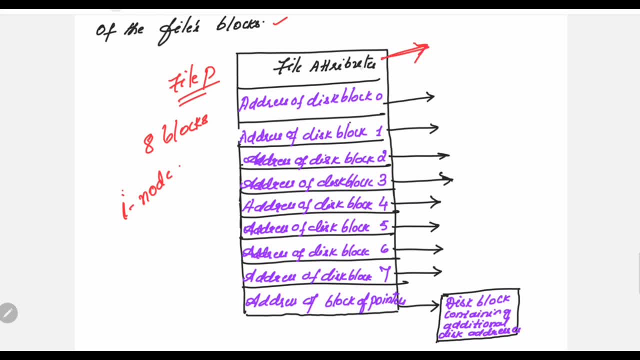 inode. So the starting part of the inode will have the attributes of the file. attributes mainly are what? the name of the file. the size of the file. when the file was created. who is the owner of the file? when was the last modification then? what are the permissions given to the? 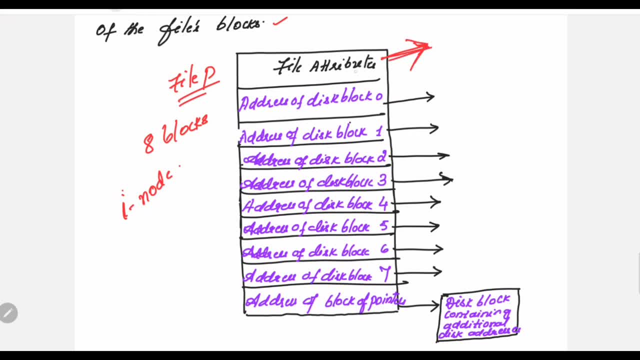 file. So like this: we have several attributes. all those attributes get stored here in the initial part of the inode. The next is what it stores: the address of each of the blocks of that file. Suppose if I am taking 8 blocks for file p. 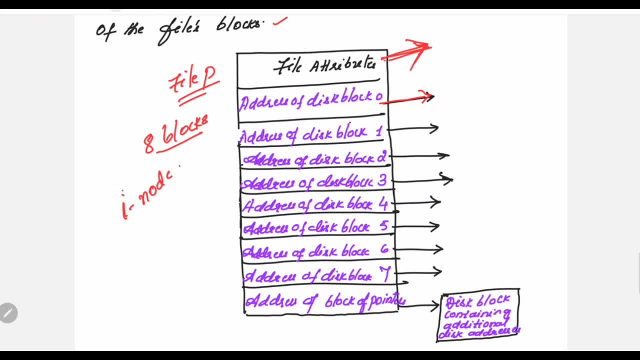 So I will have here 1, 2, 3, 4, 5., 6, 7, 8 entries. so because I am starting from 0, it will end at 7.. So this way you can try to overcome the drawback of the previous method. but how we are trying. 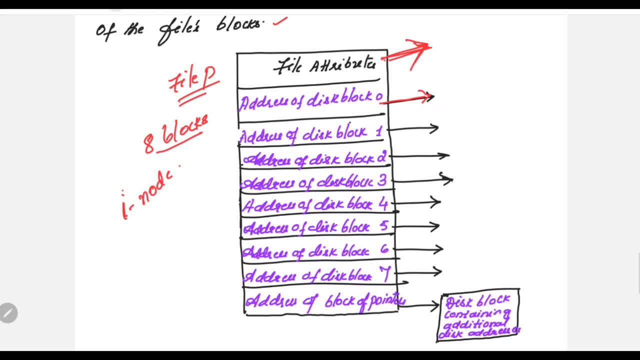 to solve. there also, we had a table which was there in the main memory. So this inode is also getting stored in the main memory. then what is the difference? the difference is this inode will not be stored in the main memory all the time, only whenever the file gets opened. so that file inode will be brought into the main memory this way you. 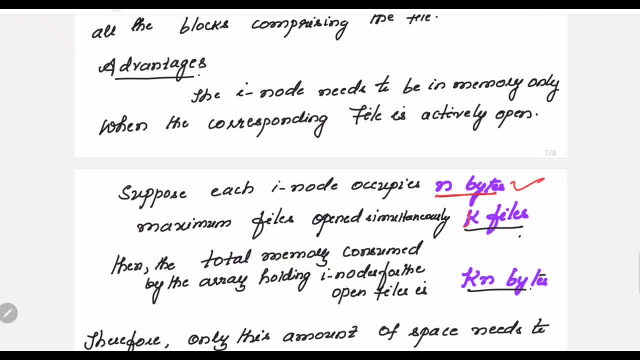 are not wasting the space in the main memory. Let us assume that k files get opened simultaneously. then the total memory consumed by the array holding inode for the open files is k into n bytes. For example, if the inode occupies 16 bytes and if you have opened 10 files at a time, 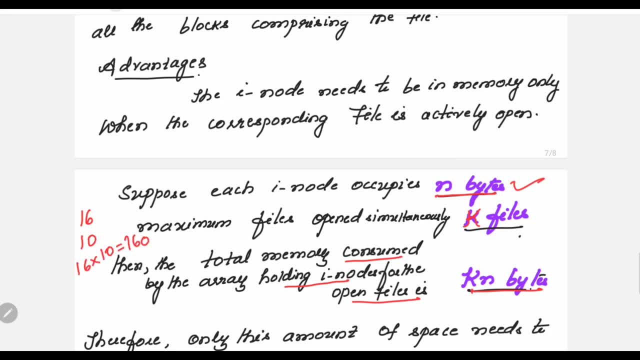 then 16 into 10. only this much, 160, 160 bytes, will be consumed by the array. So this is just an example. It cannot be so less the values, but definitely with this method you are going to save the main memory space also.